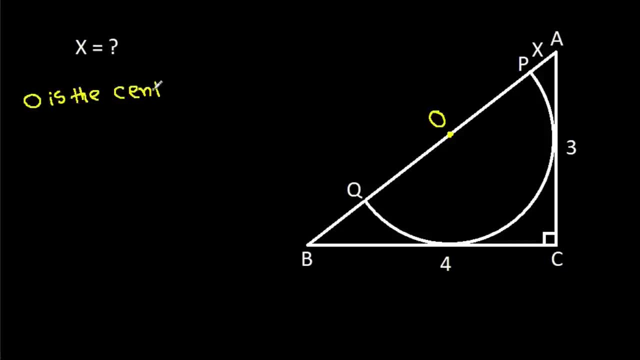 O is the center of the semicircle. Then we have BC is 4 and AC is 3.. We have BC is 4 and AC is 3.. And suppose DC, This point is D and this point is E, Then OD and OE. 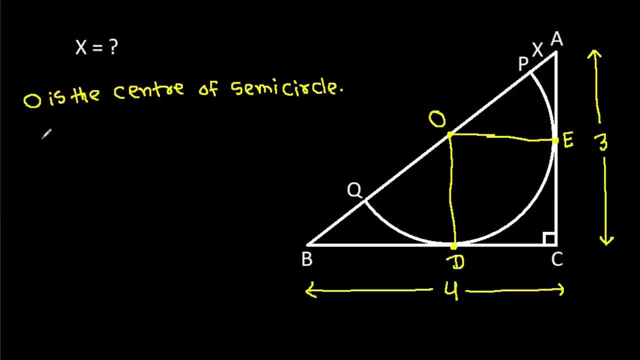 They will be radius, OD it will be equal to OE, That will be radius. Suppose R, OD is R and OE is R, And where? Here and also in any circle, radius and tangent, they are perpendicular to each other. so this: 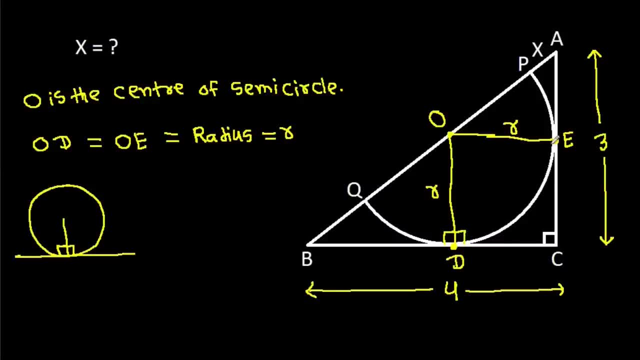 angle it will be 90 degree and this angle, it will be 90 degree. and now in ODE, this angle is 90 degrees, This angle is 90 degrees, This angle is 90 degrees. so this angle, it will be also 90 degree, and we have OE is equal to OD, that is R. 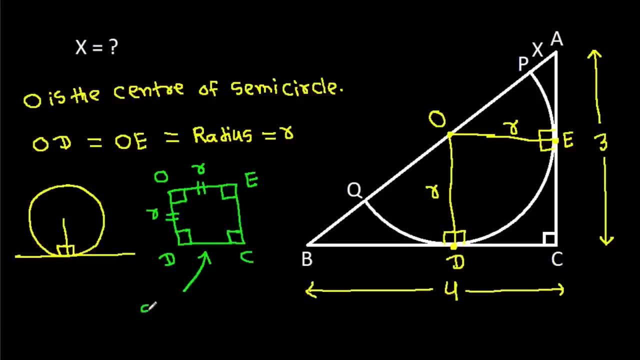 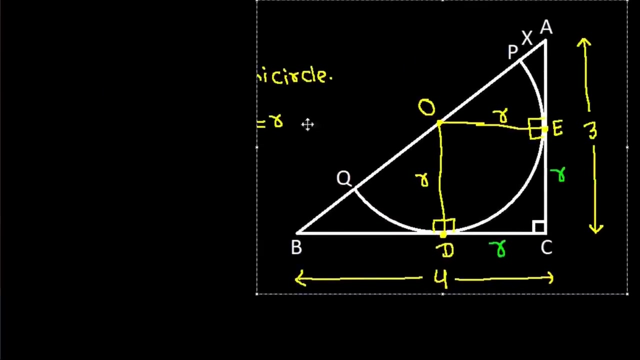 that means ODCE, it will be a square. so OE it will be equal to OD, it will be equal to DC, it will be equal to CE. that will be R. so DC it will be R and CE it will be R. and now we have: BC is 4 and BC is BD plus DC. that is 4, and it is BD plus DC is R, it is 4.. so 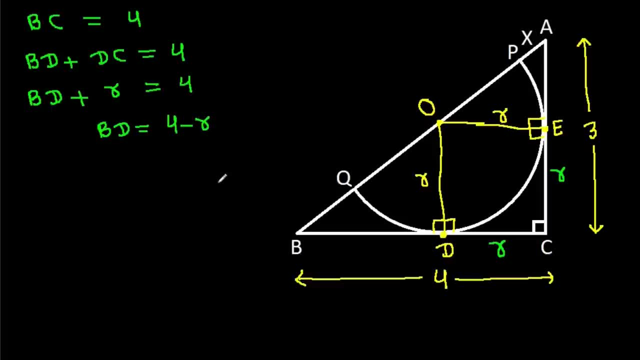 so BD it will be 4 minus R BD it will be 4 minus R, and we have AC is 3 and AC is A is plus EC, it is 3, and it is AE plus EC is R, it is 3, so AE it will be 3 minus R AE. 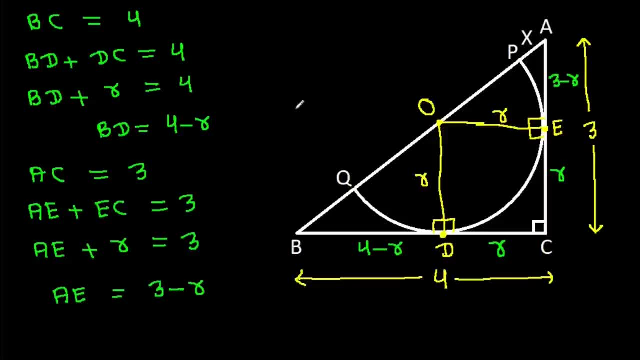 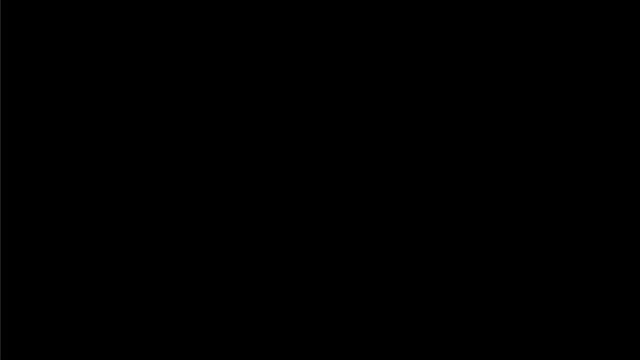 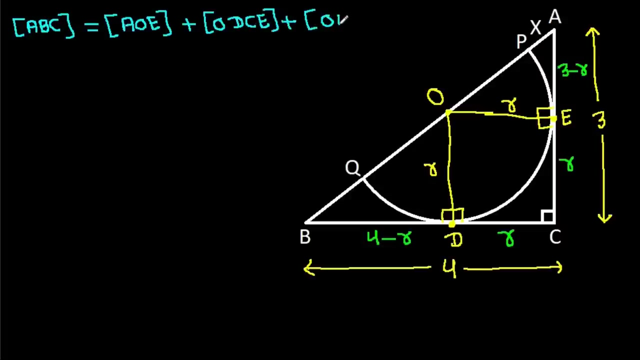 it will be 3 minus R and now area of ABC. it will be equal to area of AOE plus area of ODCE plus area of OBD and area of ABC it will be 1 by 2 times. base is BC and height is AC. it is equal to area of AOE. it will be 1 by 2 times. 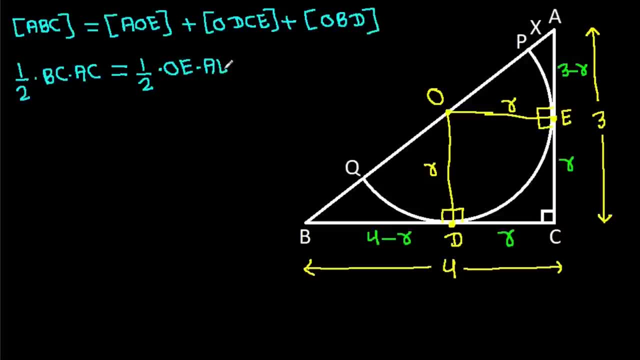 base is OE and height is AE plus and ODCE. it is square, so area of ODCE it will be DC times CE plus area of OBD it will be 1 by 2 times base is BD and height is OD And it is 1 by 2 times BC is 4, AC is 3, it is equal to 1 by 2 times OE is R and AE is. 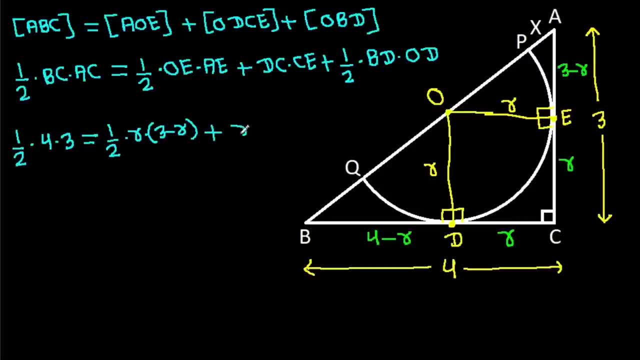 3 minus R plus DC is R times CE is R plus 1 by 2 times BD is 4 minus R times OD is R, and now 2 times 2 is 4 and 2 times 3 will be 6. it is equal to 1 by 2 times R times 3. 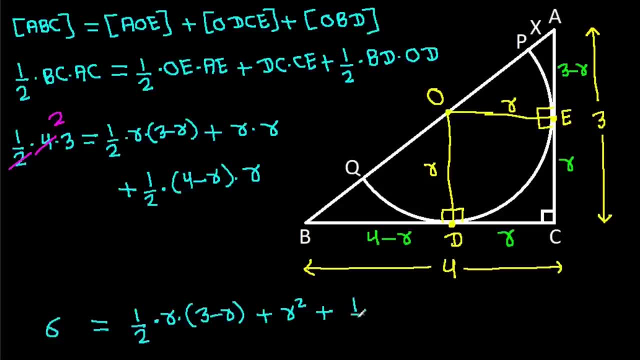 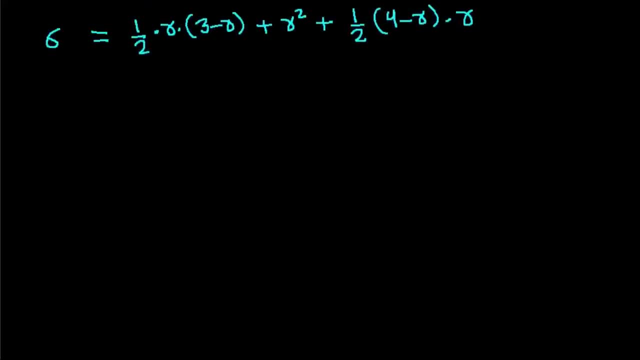 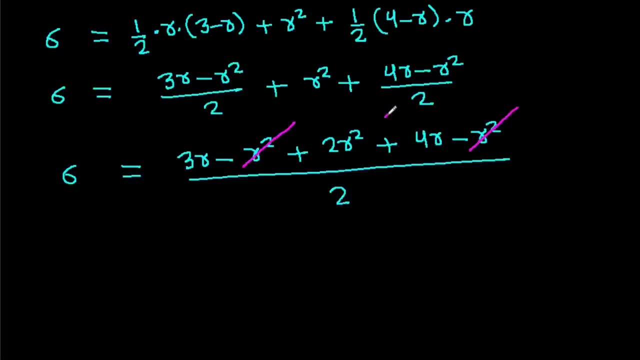 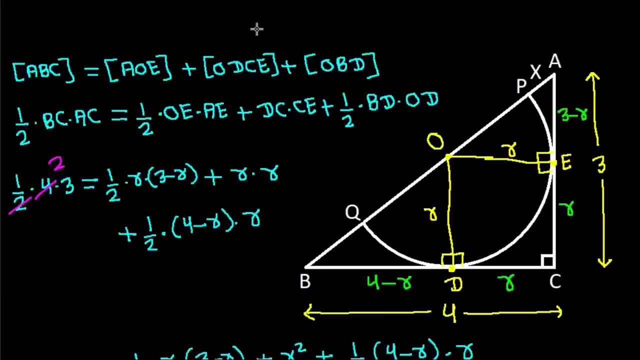 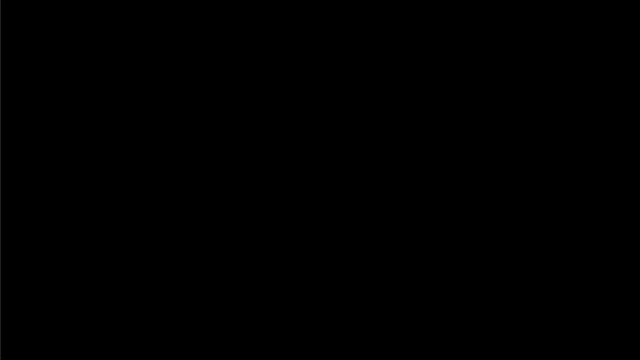 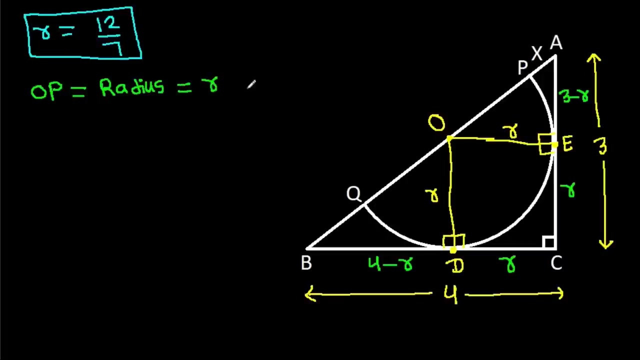 and we get: R is 12 by 7 and now OP it will be also radius, that will be R, OP will be R, and now interangle: AOE it is A AOE, OE is R, AE is 3 minus R and AO it will be R plus X. 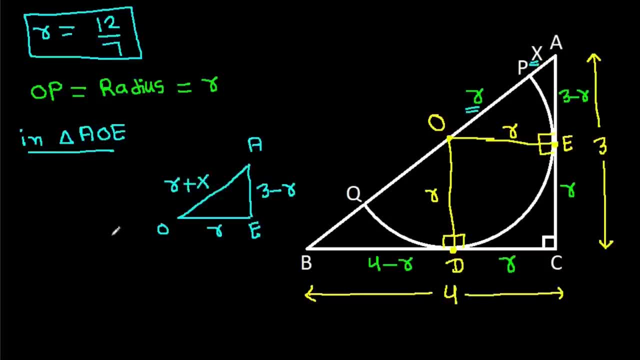 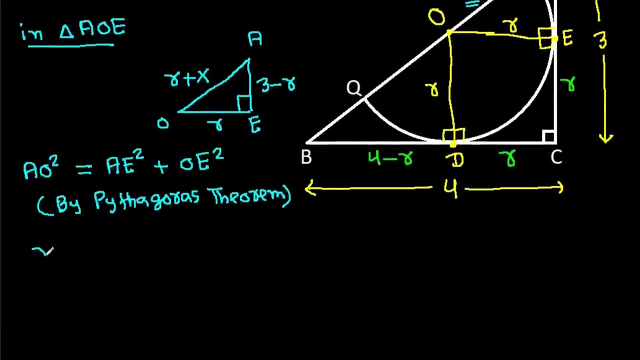 AO will be R plus X and this angle is 90 degree. so AO square it will be equal to AE square plus OE square it will be equal to 7 R minus R square by Pythagoras, Pythagoras theorem, and AO, and AO is R. 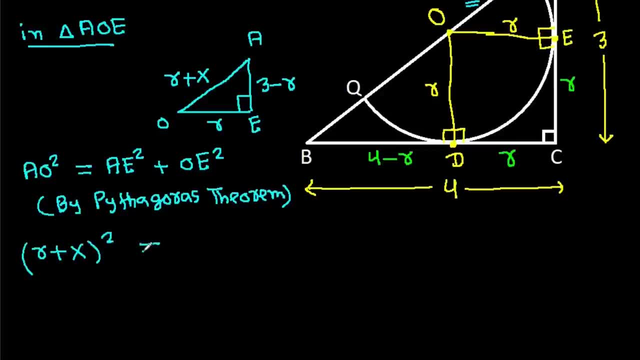 is R plus X square, it is equal to AE, is 3 minus R square plus OE r sq, and it is r sq minus x sq minus 2 times r times x. it is equal to 3 minus r sq. it will be 3 sq plus r sq minus 2 times 3 times r plus r sq and r sq will get constant. so 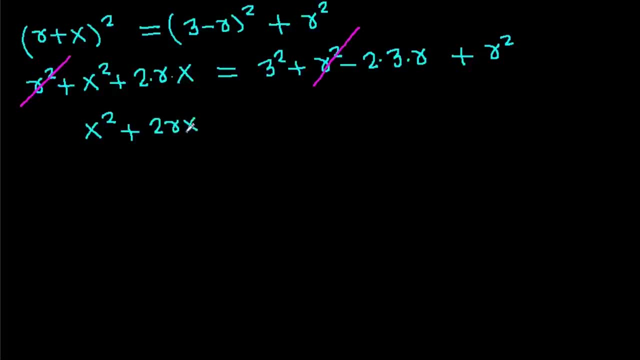 we get x? sq plus 2, rx is equal to 9 minus 6 r plus r sq and we have r is 2n by 7, so it is x? sq plus 2 times 2n by 7 times x is equal to 9 minus 6 times. 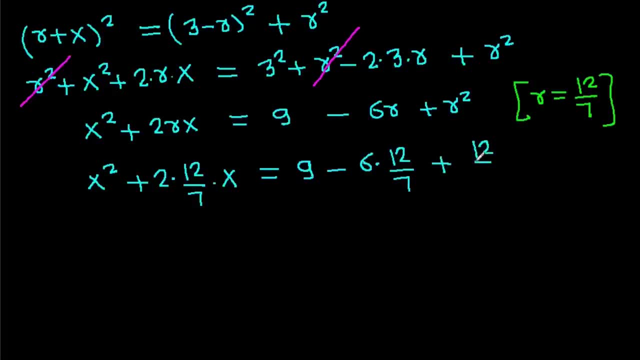 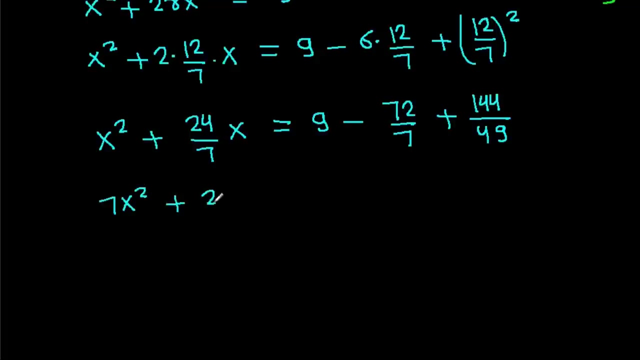 2n by 7 plus 2n by 7 sq, and it is x sq plus 24 by 7. x is equal to 9 minus 72 by 7, plus 144 by 49, and it is 7 x sq plus 24. x by 7 is equal to, and here 49 will be lcm. 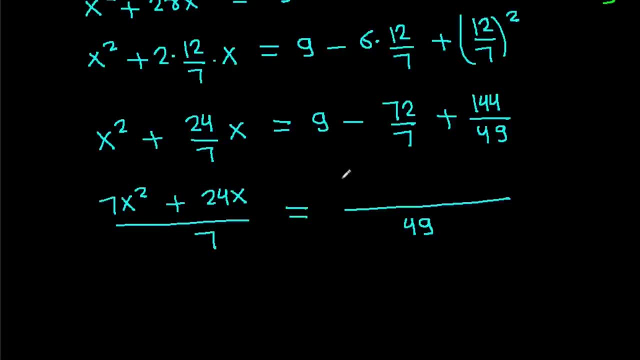 and 49 times 9, it will be 441. minus 72 times 7, it will be 504. and 7 times 7 is 49. so it is 7 x 49 is 441, and 7 x 7 is 49. 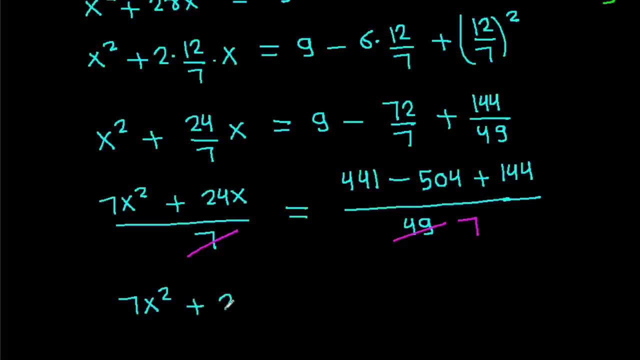 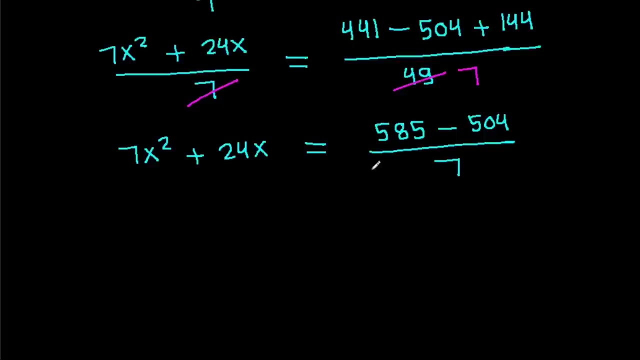 it is 7x square plus 24x, is equal to 441 plus 144.. It will be 585 minus 504 by 7.. And if we cross, multiply, then 7 times 7x square plus 24x, it will be 585 minus 504 and it is 49x. 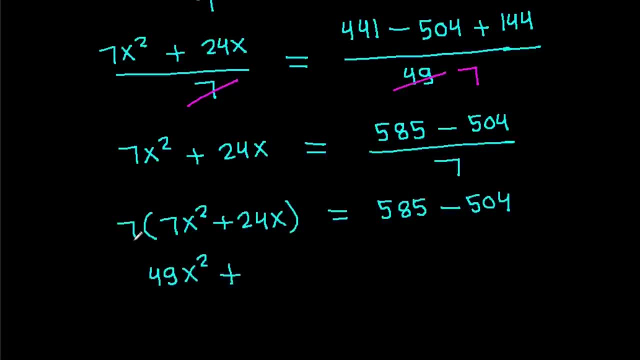 square plus 7 times 24x, It will be 168x. It is equal to 585 minus 504, it will be 81 and it is 49x. square plus 168x minus 81 is: 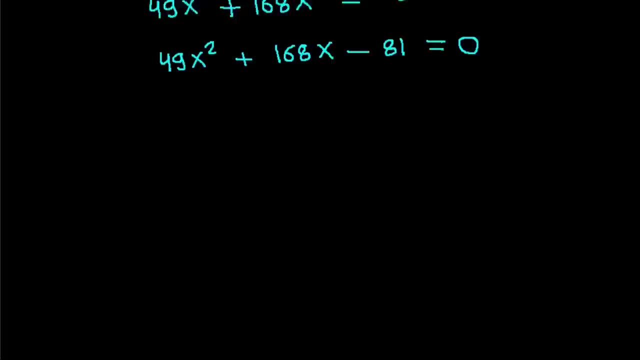 equal to 0.. And for equation ax square plus bx plus c is equal to 0, x is equal to minus b, minus minus a square root of b square minus 4ac by 2a, And here a is 49, b is 168, c is 49.. 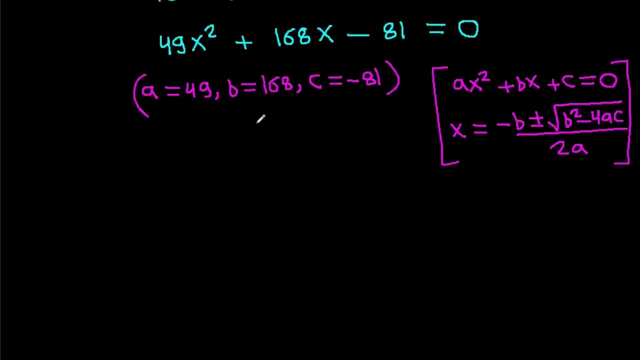 And c is minus 81. So x will be equal to minus. b is 168 plus minus a square root of 168 a square minus 4 times 49 times minus 81 by 2 times 49. Okay, And x is equal to minus 168 plus minus a square root of 168 a square and minus times minus. 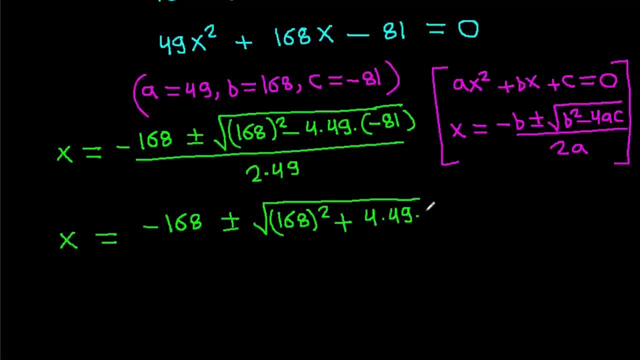 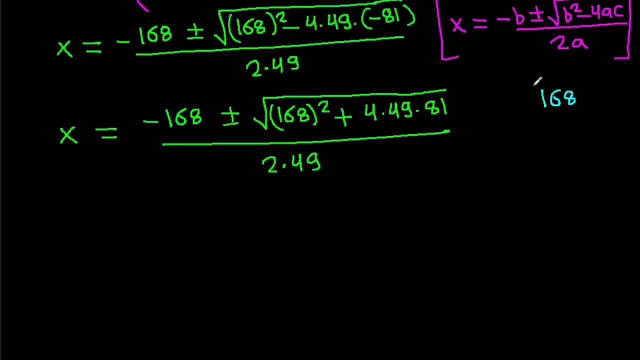 will be plus 4 times 49 times 81, by 2 times 49. And now 168, it is 2 times 84,, 2 times 42,, 2 times 21,, 3 times 7,, so 168 it is equal. 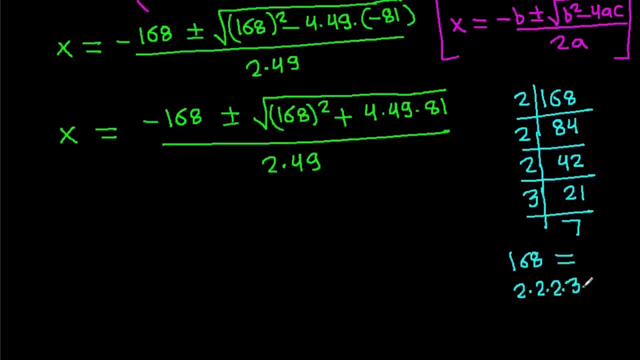 to 2 times 2 times 2 times 3 times 7.. Okay, So 168 is equal to 2 times 2 times 2 times 3 times 7.. Okay, So x will be equal to minus 168, it is 2 times 2 times 2 times 3 times 7, minus minus. 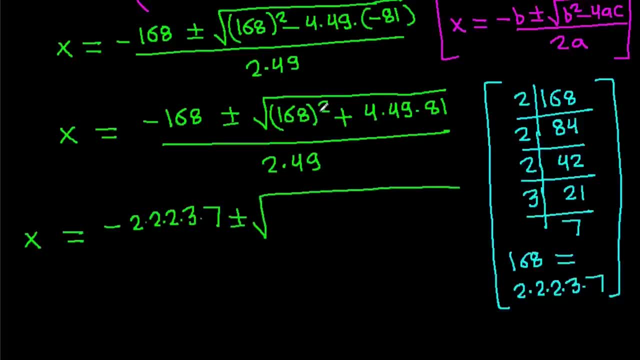 a square root and 168 a square, it will be 2 a square times 2 a square times 2 a square times 3 a square times 7 a square. Okay So, 168 plus minus 4 is 2 a square and 49 is 7 a square times 81 is 3 a square times. 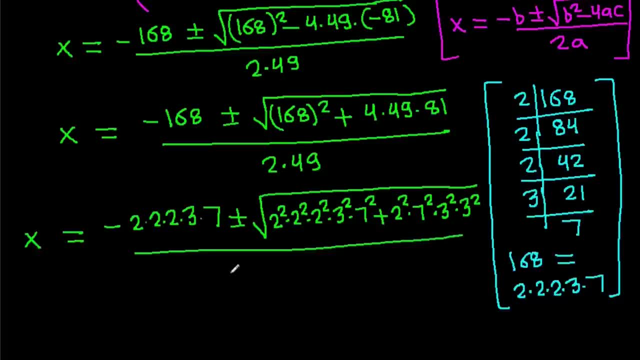 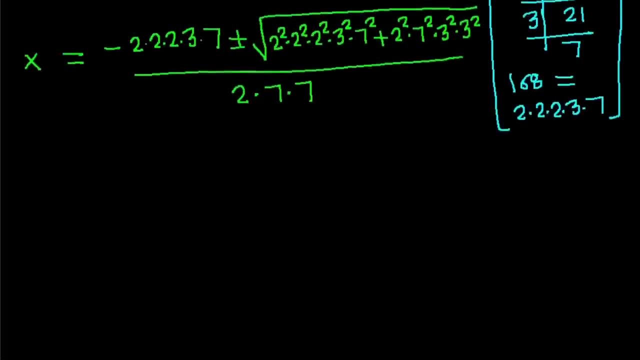 3 a square by 2 times 49 is 7 times 7.. And x will be equal to minus 2 times 2 times 2 times 7.. Okay, So x will be equal to minus 2 times 2 times 2 times 7.. 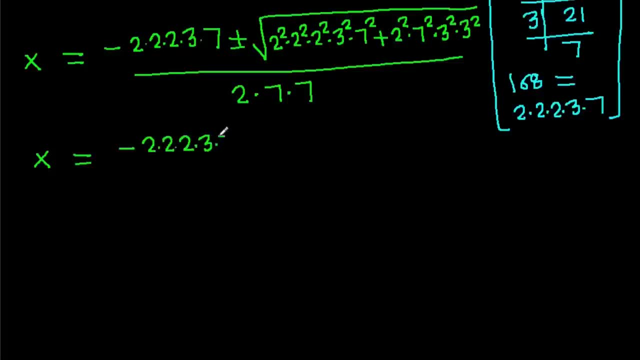 Okay, So x will be equal to minus 2 times 2 times 2 times 3 times 7, plus minus a square root, And here we can take 2 a square times 3 a square times 7 a square common. 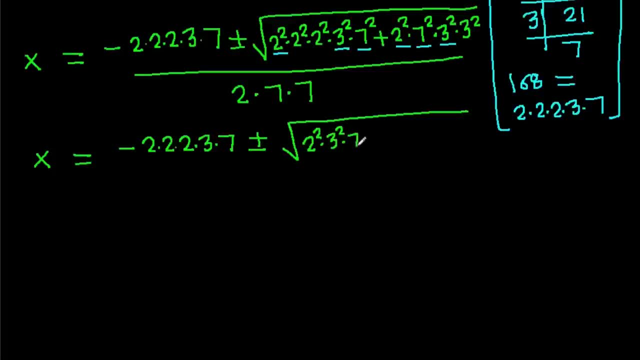 We can take 2 a square times 3 a square times 7 a square common and it will be 2 a square times 2 a square plus 3 a square By 2 times 7 times 7, so x will be equal to minus 2 times 2 times 2 times 3 times 7 plus. 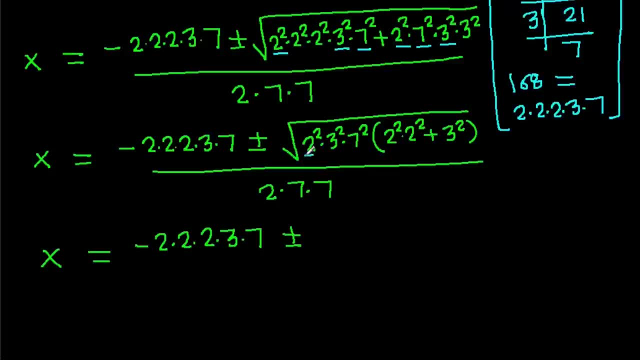 minus and a square root of 2 a square times 3, a square times 7 a square, it will be 2 times 3 times 7 times a square root. Okay, So x will be equal to minus a square root and 16 plus 9, it will be 25 by 2 times 7. 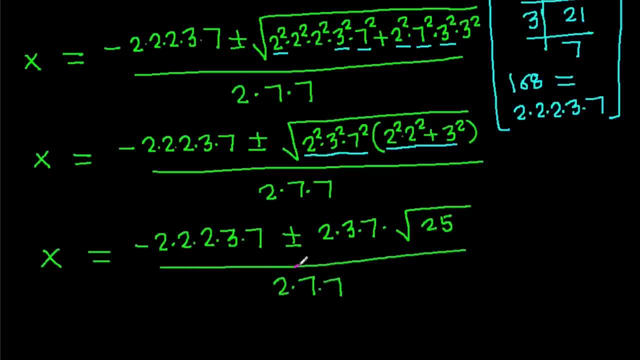 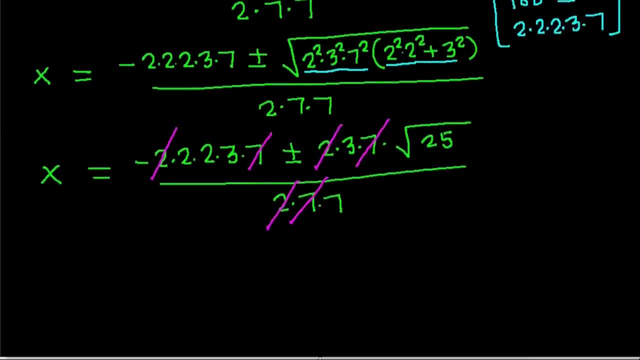 times 7 and 2 will get cancelled and 7 will get cancelled. So x is equal to minus. Okay, So x 2 times 2 times 3 will be 12, plus minus 3 times 5 will be 15 by 7.. 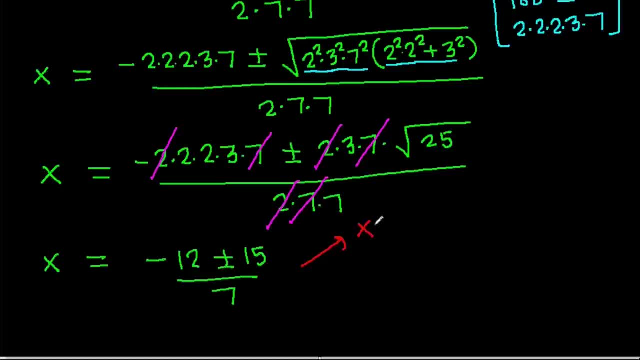 So from here we get x is minus 12 plus 15 by 7, and we get x is minus 12 minus 15 by 7. And this is negative. So it is not possible. and from here it is 3 by 7.. 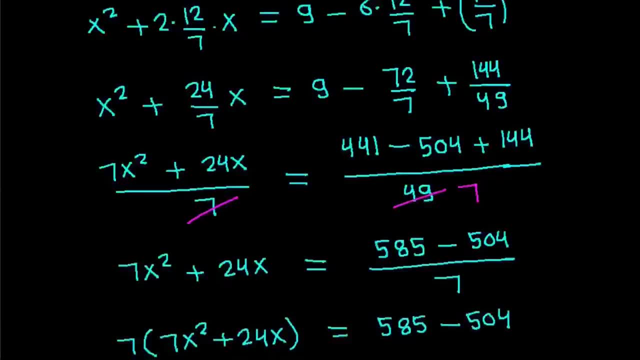 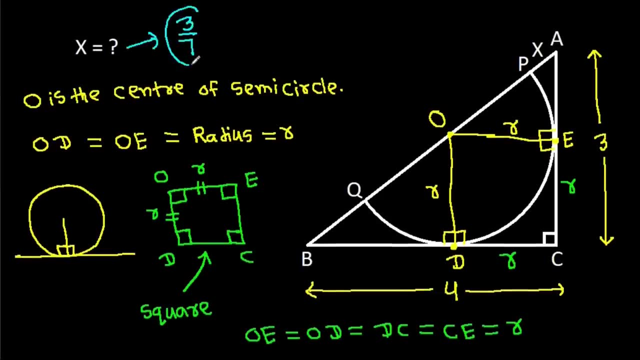 So x 2 times 2 times 3 will be 3 by 7..